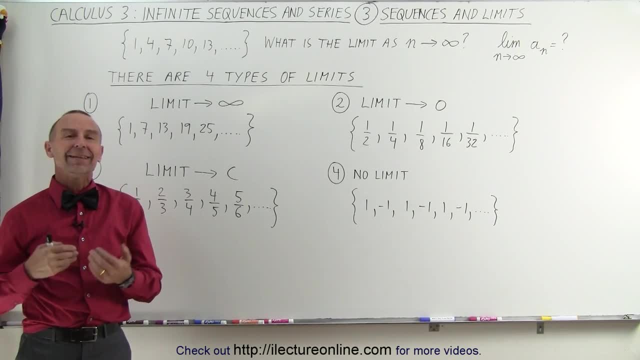 Welcome to our lecture online. Now let's talk about the limits of a sequence. What happens if we continue adding more and more numbers to the sequence- and essentially, a sequence has an infinite number of numbers. typically, In this case, you can see that the numbers keep on increasing. 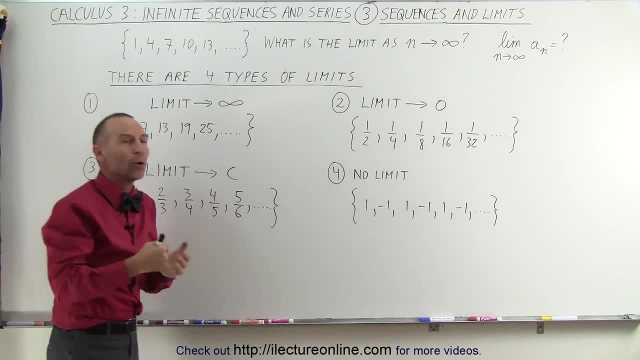 The question is: what would be the final number, so to speak, if we go all the way to the very last number in the sequence? Well, what is the last number in the sequence? Well, the last number is in the sequence is when the number n, the nth value of the sequence, becomes infinite. 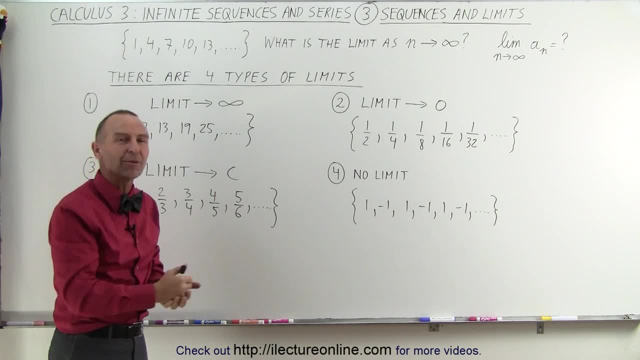 So, in a way, there really isn't the last number of the sequence. There's always one more after that and one more after that. But where is the sequence going? What will be that last value? What does it converge to if it just kept going the way it was? Well, in some cases there is. 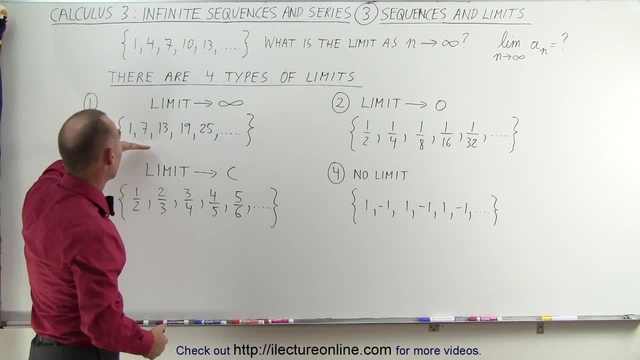 actually no limit, It just keeps increasing. In this case, we have an arithmetic sequence here Where you can see that the next value is always six larger than the previous value, And if this goes on forever, for the nth value when n goes to infinity- in the limit, of course. 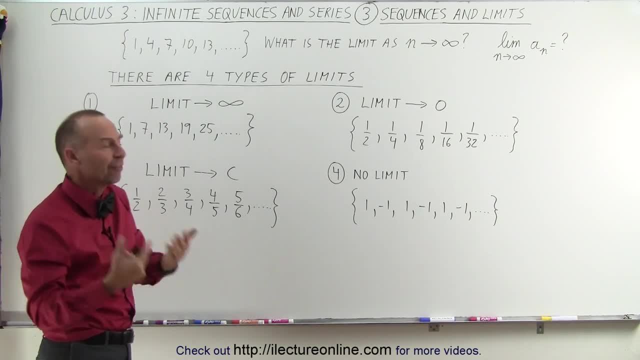 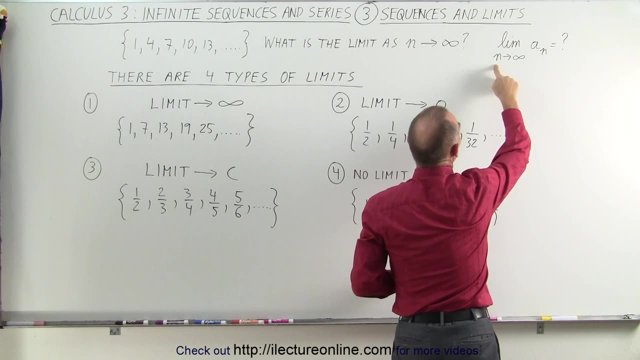 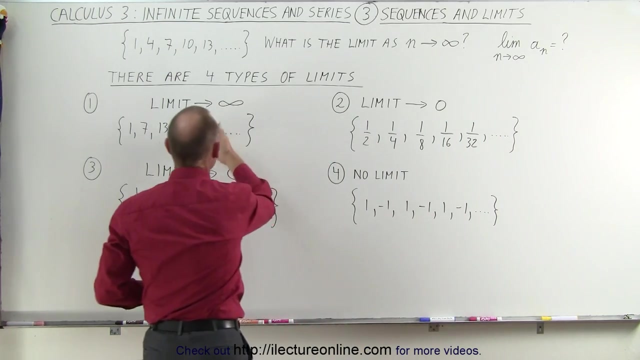 this goes to infinity. There is no such real limit. The limit is infinity for this particular sequence. The way we write that mathematically is as follows: The limit as n goes to infinity of that particular element in the sequence, a sub n is equal to, and you can see that if it keeps on, 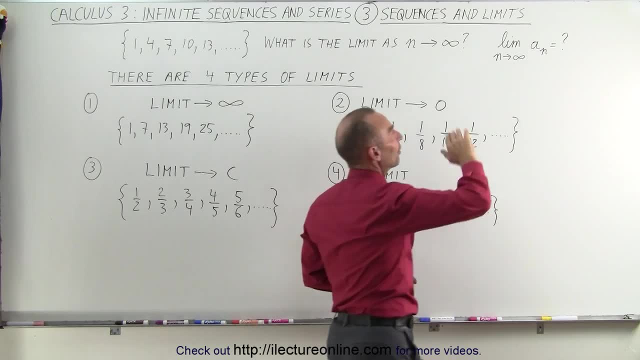 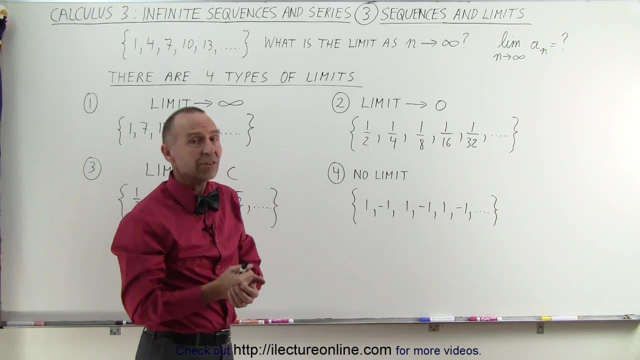 increasing, Then of course that will go on to infinity, and the very last one in the sequence as n goes to infinity will. of course that will be infinity, But in some cases the limit goes down to zero. The limit goes down to zero if, for example, the numerator stays as a constant value and the 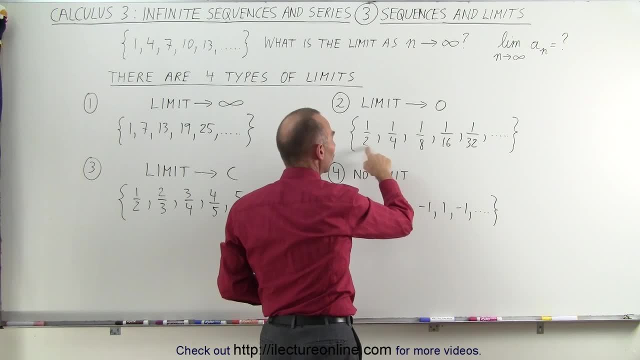 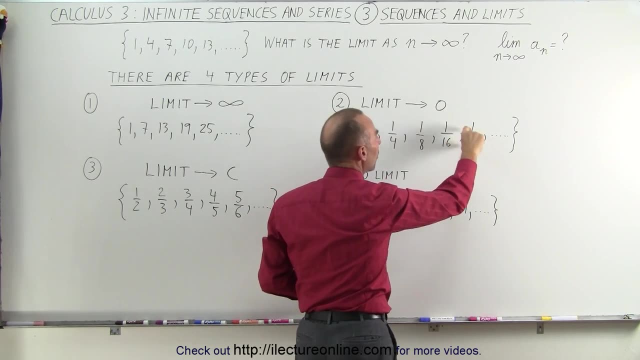 denominator is double what it was before. So this one is four instead of two, This one is eight instead of four, and so forth. You can see that the number in the sequence gets smaller and smaller and smaller, and if this keeps going on forever. 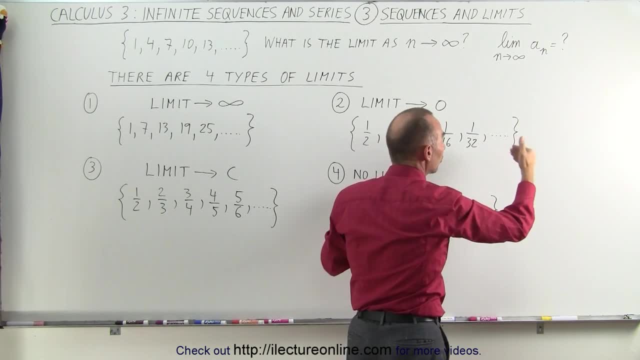 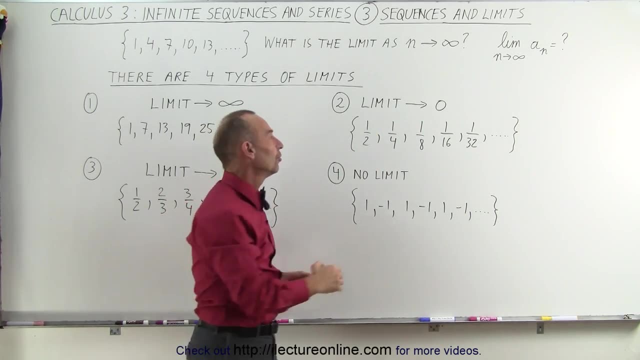 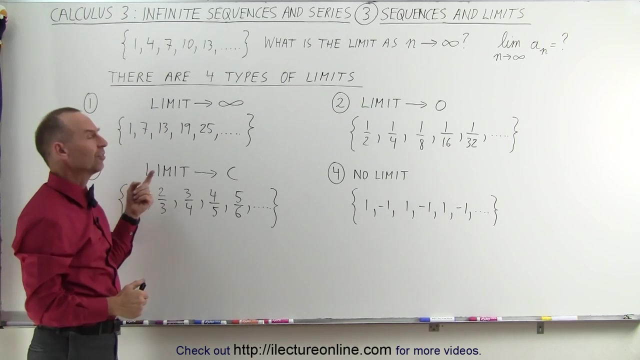 You can see that the bottom will get larger and larger and larger, and in the limit the denominator will go into infinity, and one divided by infinity is indeed zero. So you can safely say that in this case the limit of this sequence is zero. Sometimes the limit of a sequence becomes a constant or 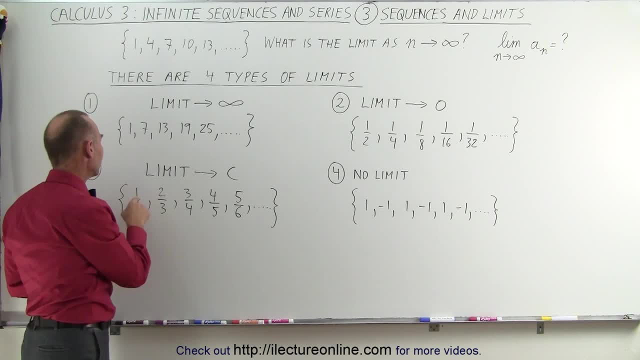 converges down to a constant. Here you can see that the numerator increases by one and so does the denominator, except the denominator started as a two and the denominator is a three, So the denominator is a two. The numerator started as a one, So you can see that this is one-half, this is two-thirds, this is: 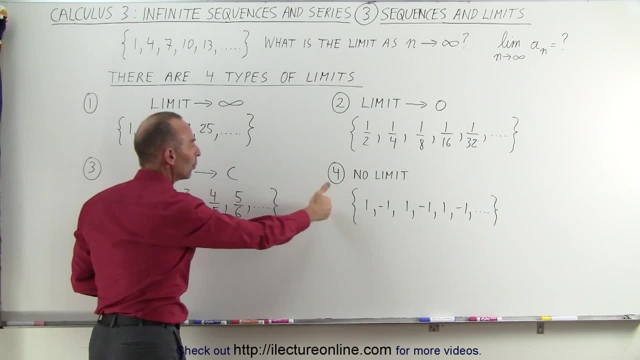 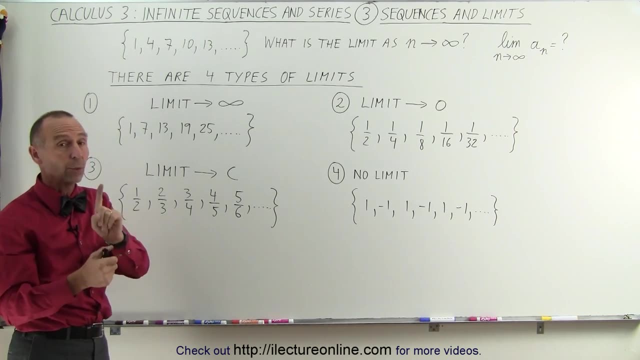 three-quarters, this is four-fifths, and as you continue progressing with this sequence, you can see that the ratio of the numerator to the denominator becomes closer and closer and closer to the value, one which is a constant, And so, in the limit, as you go to the nth value, as n approaches infinity. 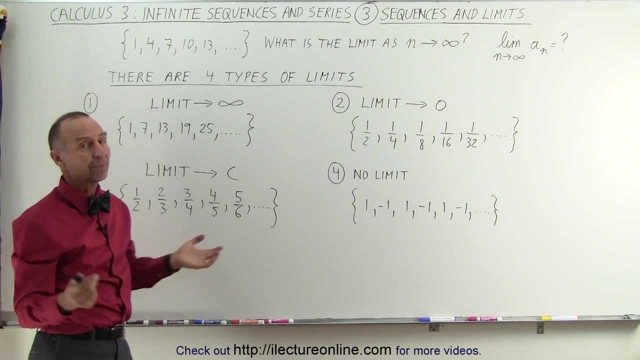 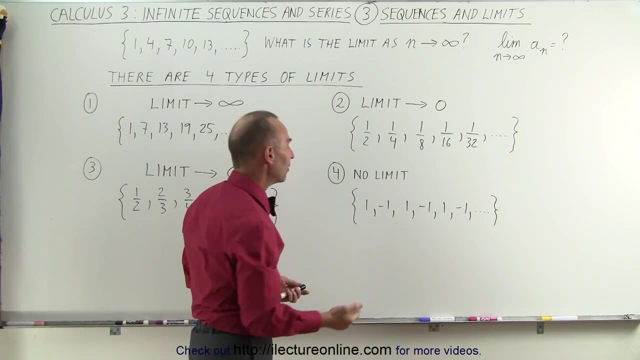 this limit will then converge to a one. In some cases, there simply is no limit. You can go on to infinity and you can see that it does not converge to a single number. The very classic cases where you keep popping back and forth between a plus one and minus one, plus one, minus one, plus one minus one, and so. 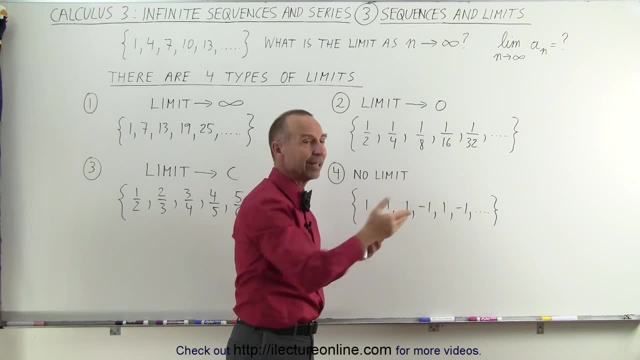 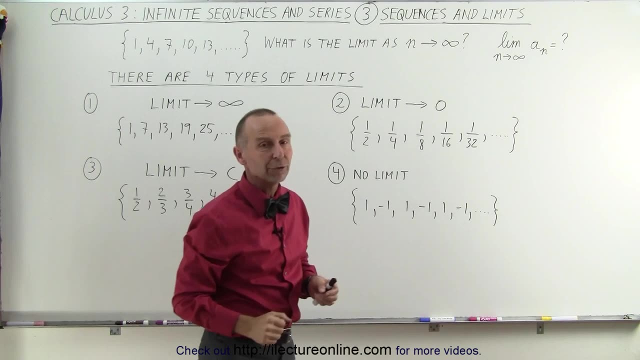 forth. you can see that no matter how long you keep going, you can do this forever- it'll never converge to a single number. So in this case there is no such thing as a limit, as you go on to infinity for the numbers in the sequence. So the four general cases you're going to get into is: 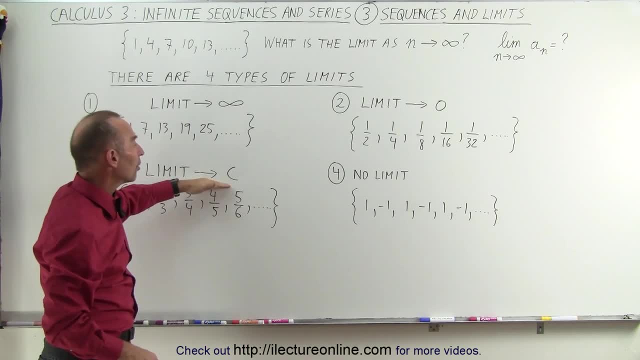 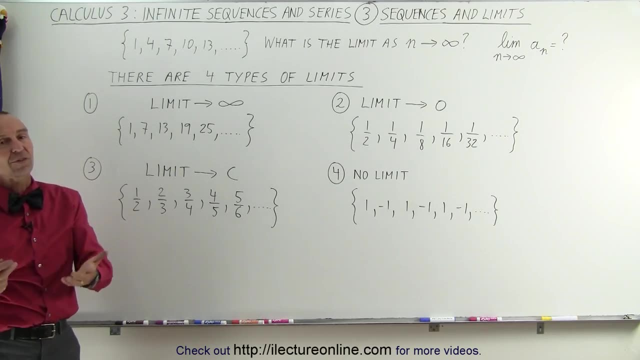 the limit is infinity, the limit is zero, the limit is some constant number and the number is zero, or there is no limit at all. And those are some of the basics as far as finding the limits of a sequence, and we'll see some examples of that as well. 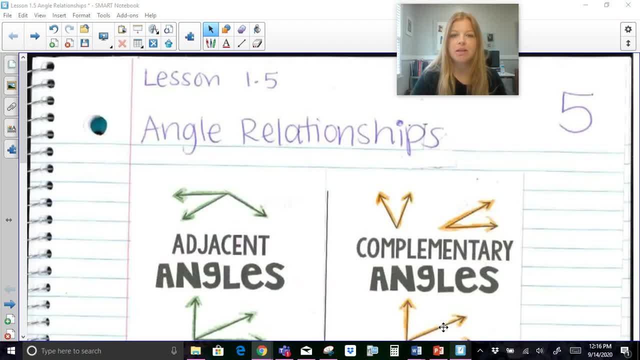 Hi everyone, welcome to this video where today we're talking all about angle relationships. So I have six very special angle relationships that I need to show you today. Make sure that, as I'm showing you each one, you're really noticing the difference between each one.